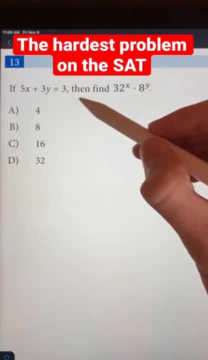 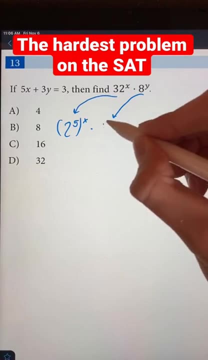 Let's see if you can do the hardest problem on the SAT. If 5x plus 3y equals 3, then find 32 to the x times 8 to the y. So the first thing I'm going to do is rewrite 32 as 2 to the power of 5, and I'm going to rewrite 8 as 2 to the power of 3.. 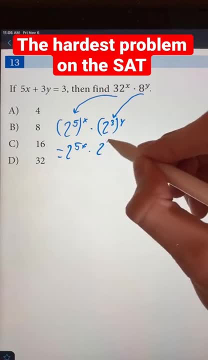 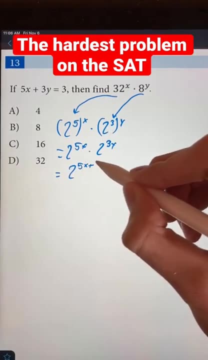 So this is just 2 to the 5x and this is 2 to the 3y, And anytime you have two exponents with the same base being multiplied together, you can just add their two exponents. So this is just equal to 2 to the 5x plus 3y and it gives us what 5x plus 3y is. 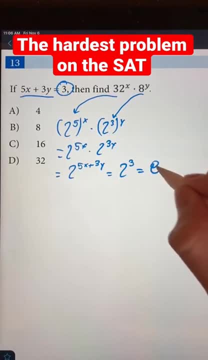 They say it's equal to 3.. So this is just 2 to the power of 3, which is just 8.. Thank you. 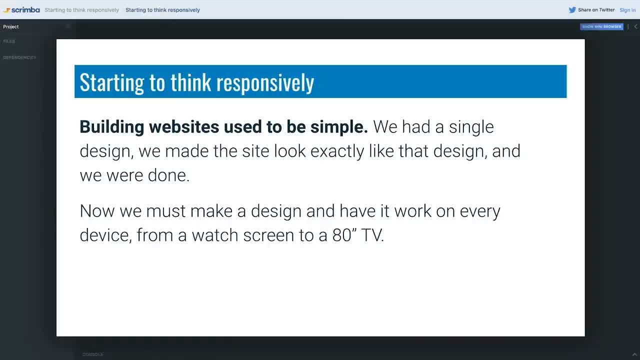 Building websites used to be simple. We had a single design. We had to make the site look exactly like that design, and then we were done. Now there's some problems with that. Browsers used to render things differently, but at the end of the day, we just had this one layout to do. It was 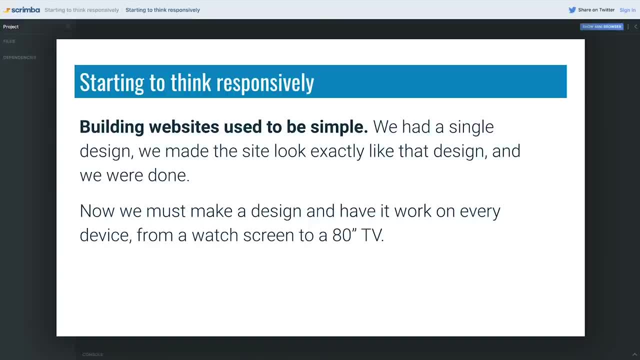 completely static. We just had to recreate what probably a photoshop document that we were given looked like, and that was it. Now we have to take a design and we have to make it work on every device, from sometimes a watch screen up to an 80 inch television. That's not necessarily something. 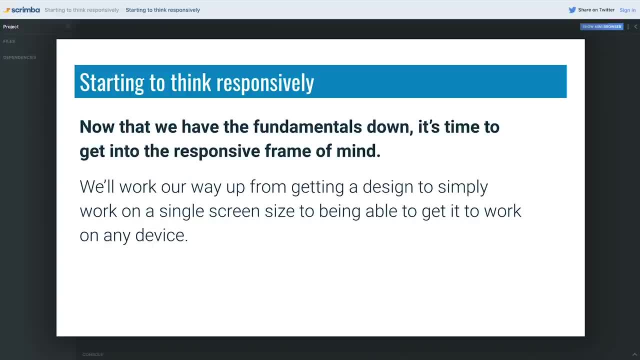 that's super easy to do, but we have the fundamentals down. We understand how to make a static site. so it's time to get into the responsive frame of mind and we're going to work our way up from getting a design to simply work on a single screen size to being able to get it to work on. 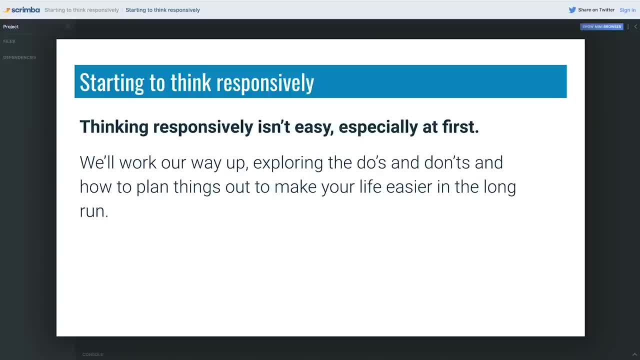 any device. Thinking responsively isn't easy at first, but we are going to work our way up. We're going to be exploring the do's and don'ts and we're going to look at how we can plan things out to make our life a little bit easier in the long run. But do know this is just an introduction to 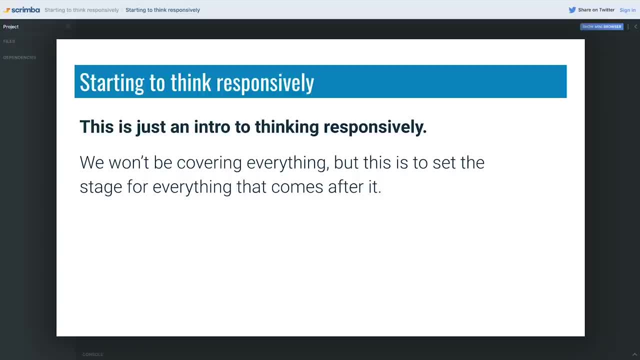 thinking responsively. We're not covering everything there is in this module about how to build a responsive website. We're getting our feet wet with it. We're going to start looking at a few new things, but I don't want to overwhelm. As I've said before, I like teaching through.